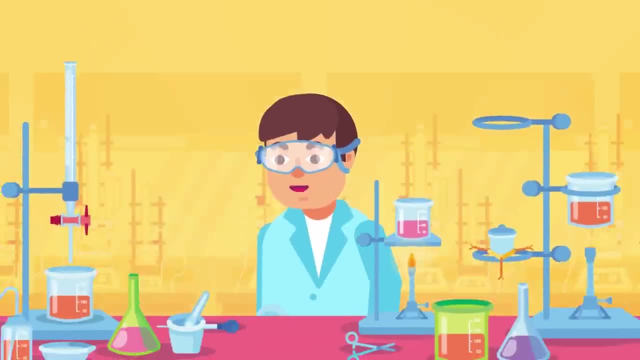 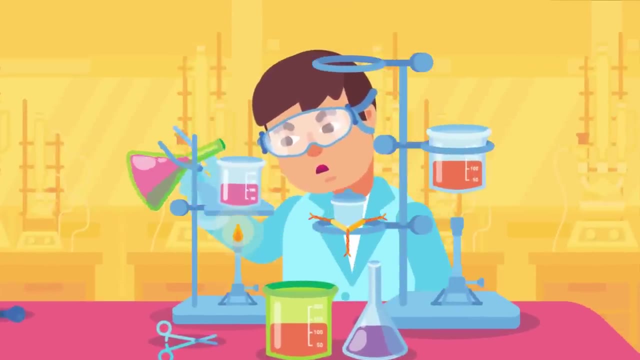 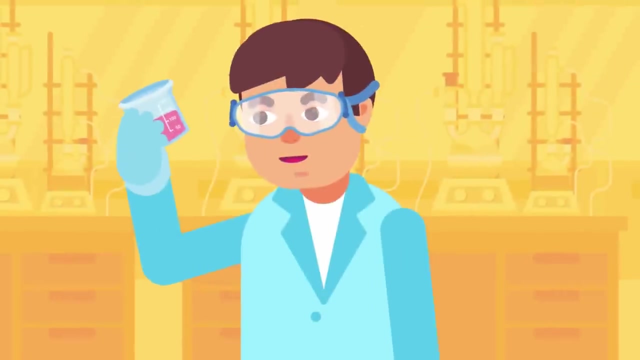 This not only makes you look cool and makes you feel like a responsible scientist, but also protects you from all kinds of chemicals you may be coming into contact with knowingly and unknowingly. Electronic balance Used for measuring mass of a substance or chemical usually consists of a pan on which you can place the substance you want to measure. 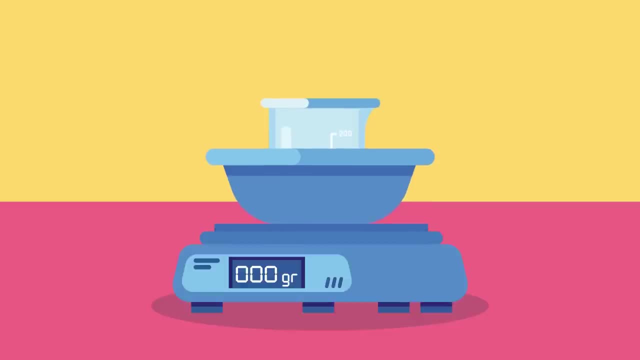 This generates current proportional to the displacement of the pan due to the pull of gravity, which then translates into the displayed reading. The electronic balance is a simple yet easy-to-understand and one of the most important equipment that should be present in any laboratory. 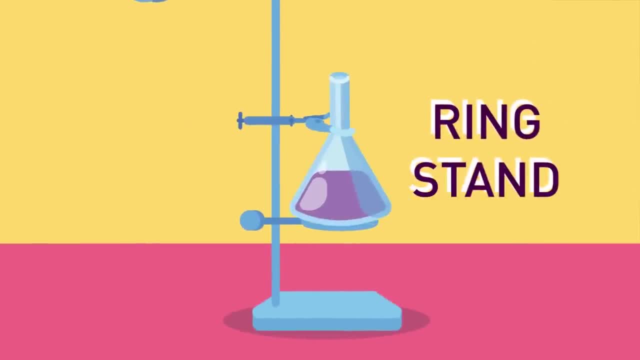 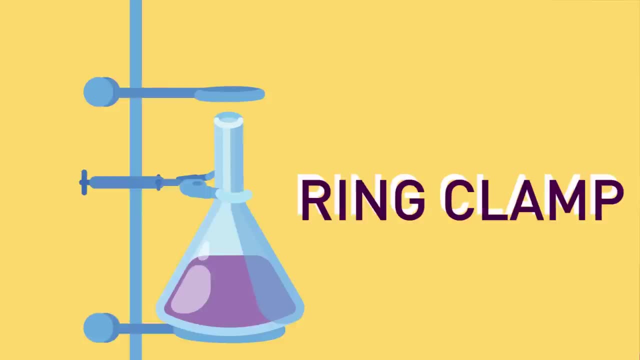 Ring stand Used as support to clamp laboratory glassware and other equipment in place so it does not fall down or come apart. Ring clamp Used with a ring stand to hold glassware such as a beaker or a funnel Wire gauze. 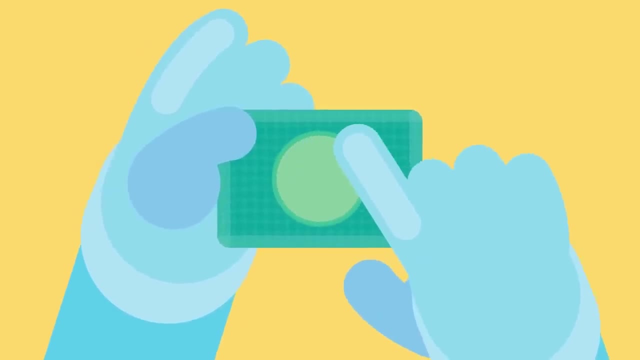 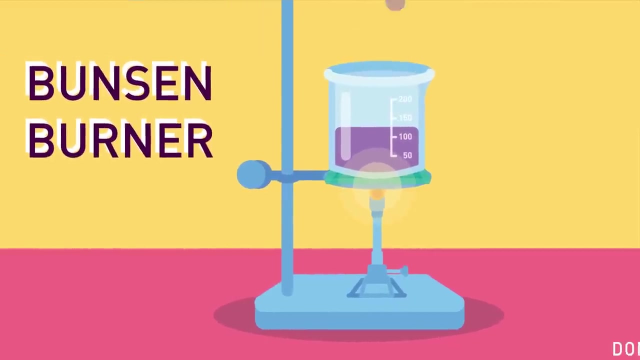 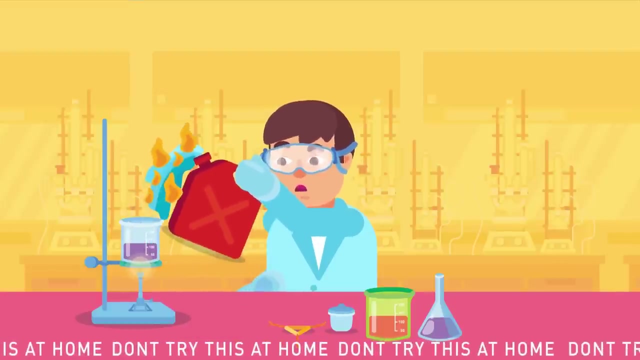 May have a fiberglass or ceramic center Used to support a container such as a beaker on a ring stand while it is being heated. Bunsen burner, Be careful not to put flammable materials like a cloth or chemicals like aromatic compounds such as petrol, anywhere near it, or this may erupt a fire. 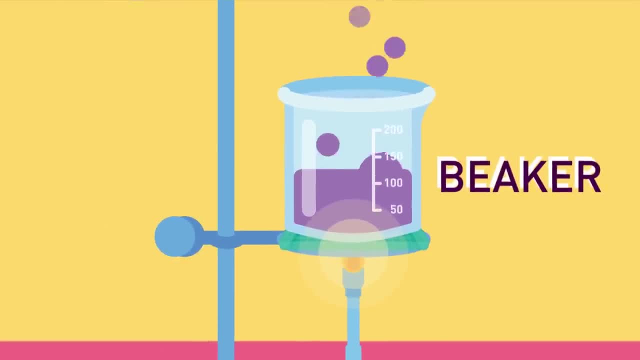 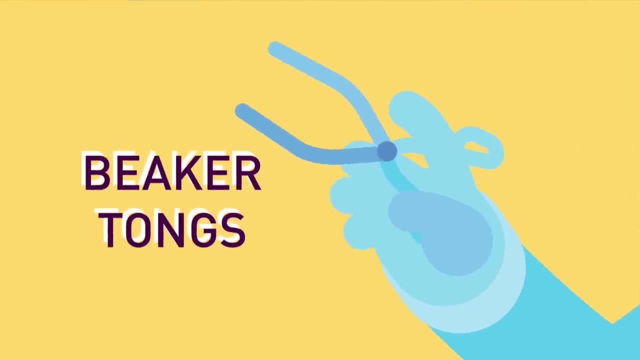 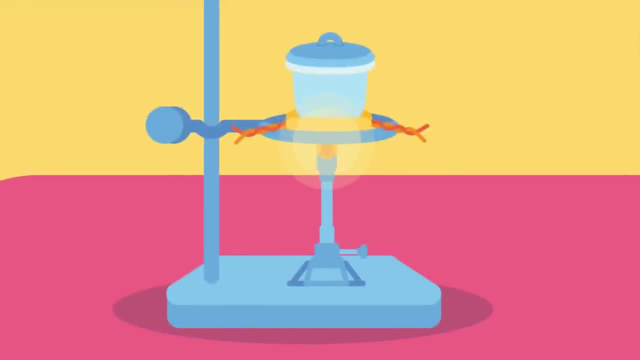 Beaker: A beaker is a glass apparatus used to hold mix and heat liquids. Beaker tongs: Metallic and looks like a scissors' older sibling. Beaker tongs is used to handle beakers. Crucible: A ceramic pot used for holding chemicals during heating. 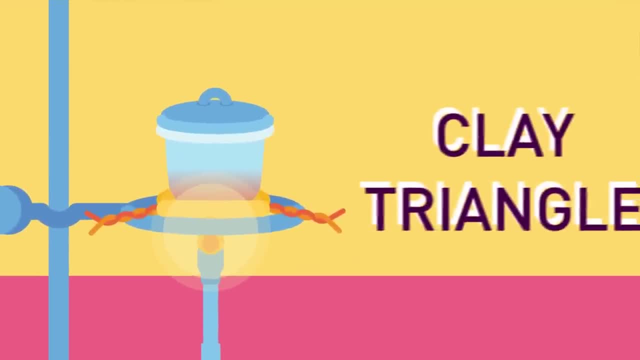 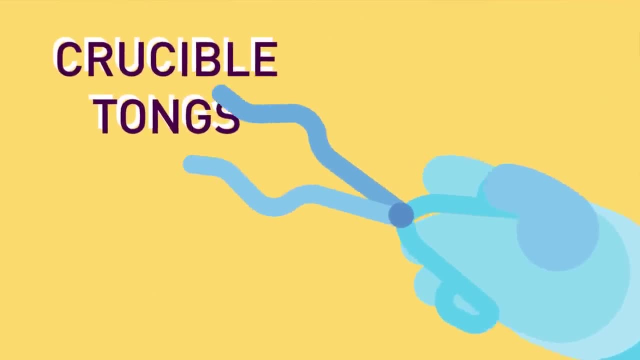 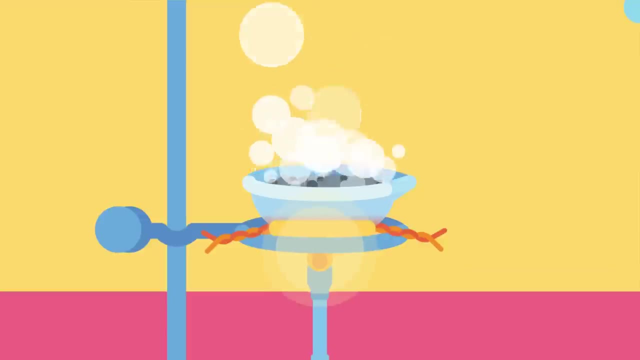 at very high temperatures. Clay triangle: A metallic triangle used to support a crucible during heating. Crucible tongs Used to hold crucibles. Evaporating dish: A wide ceramic dish used to heat liquids for evaporation. Utility clamp: A metallic clamp used to secure glassware to a ring stand. 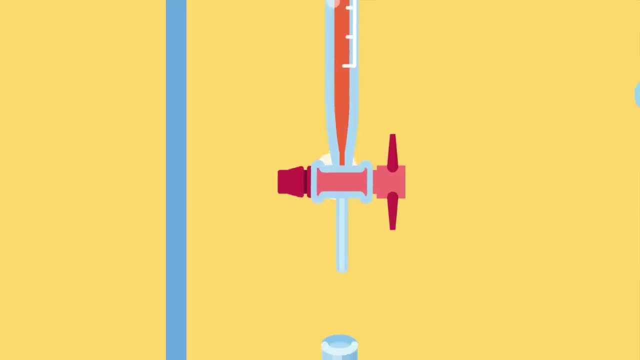 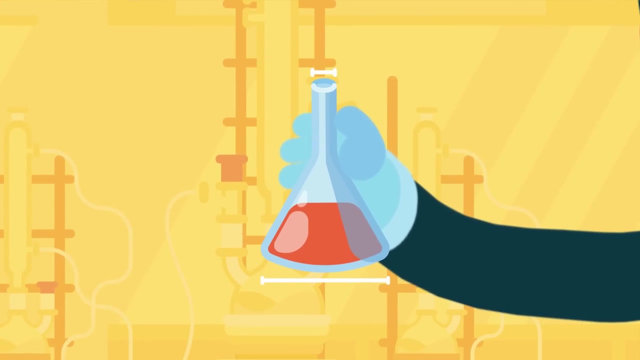 Burette- A long glass graduated tube with a tap around it. A burette. A burette is used for dispensing an accurate volume of a liquid and measuring its discharge. Conical flask, Also known as the Erlenmeyer flask, is a glassware that has a narrow neck that expands towards its base.